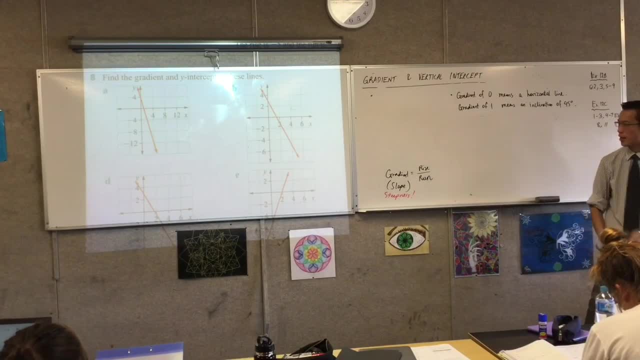 But some of you are still kind of struggling with them, so let me show you how these work. The question is: find the gradient of y intercept in these lines. I'm just going to focus on gradient for now. I think most people read off the y intercept. It's no big deal, okay. 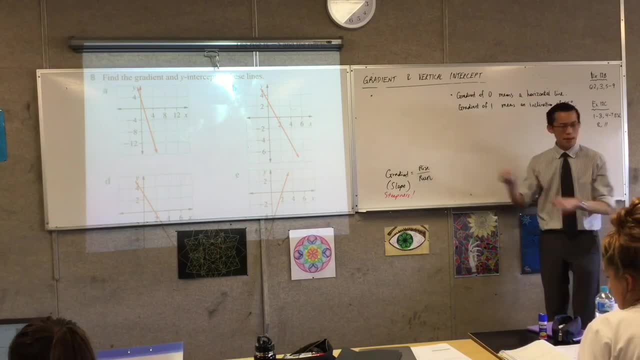 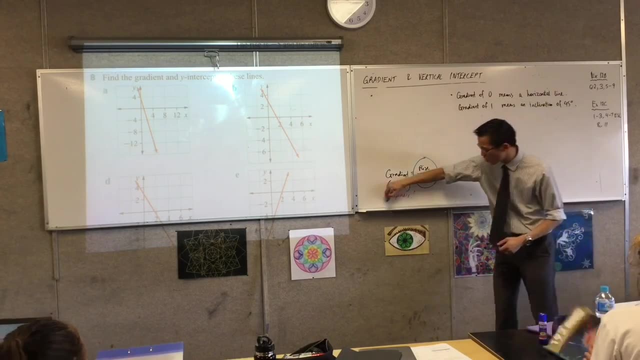 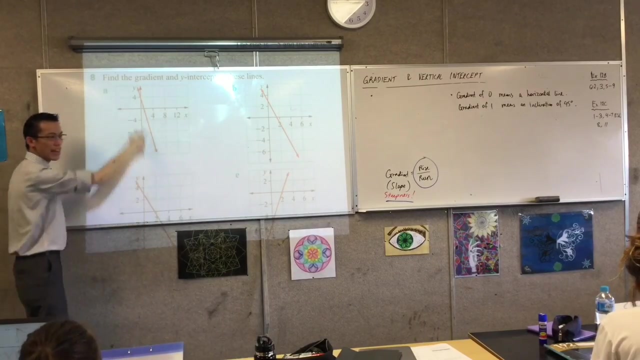 For gradient, things are a little more complicated. I just want you to remember what gradient is. Gradient is calculated by doing rise over run, but what it means is steepness. Like how steep is something? Is it shallow? Is it really? really? you know? what kind of behaviour is this line doing? 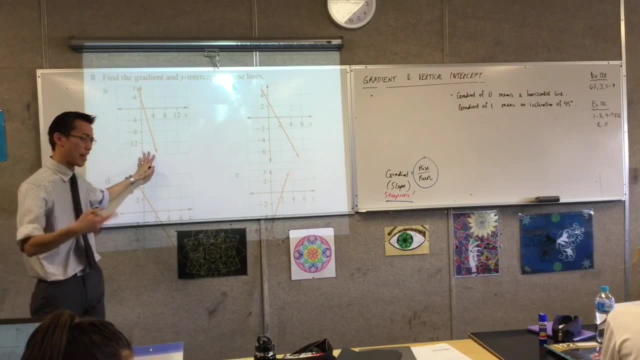 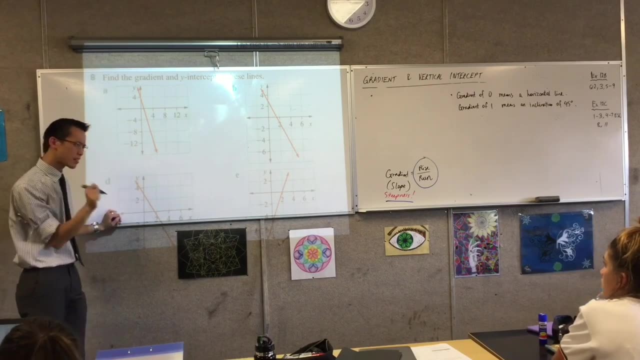 Now, do you notice? this is all about this entire topic. AM2, is about linear relationships. They're called linear because they're straight lines. okay, Now, being that it's a straight line, that means that the steepness doesn't change. 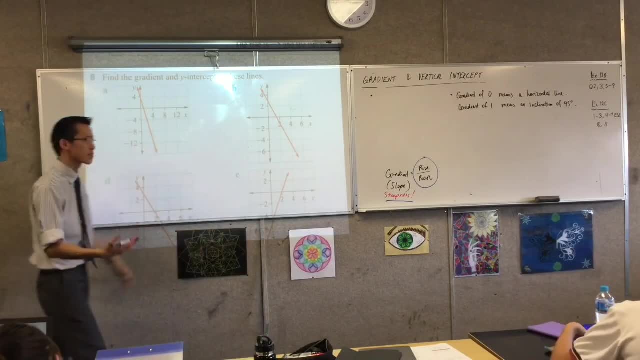 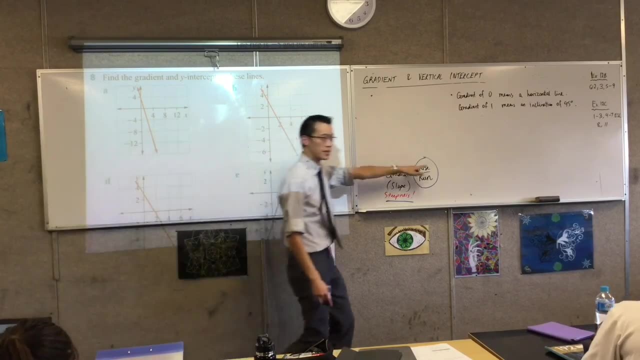 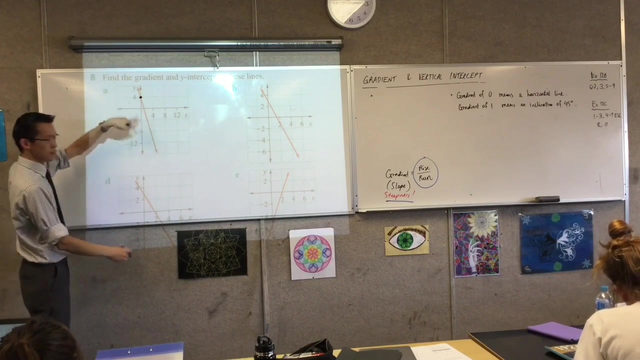 It stays the same all the way through the line. Does that make sense? So I should be able to compare any points I like on this line: do this rise over run business, and that will give me a gradient. So on ones like this, it's easy because I can pick a point here which is on like a nice grid line, and I can pick one here. 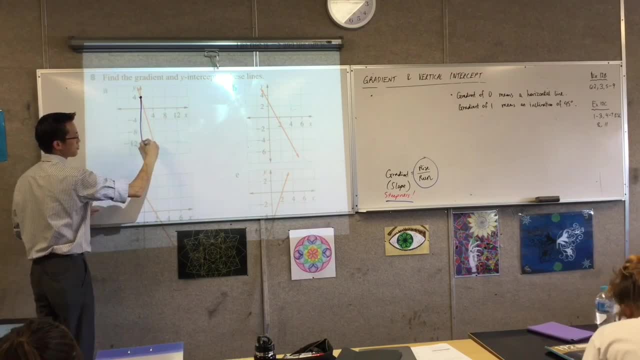 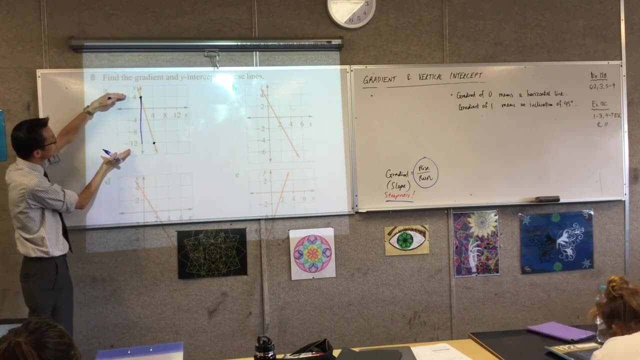 And I can see. alright, here's the rise. It goes down, Since it goes down from 4 to negative 12,. what is this length? This is 16, right, But it's negative because it's dropping. Does that make sense? 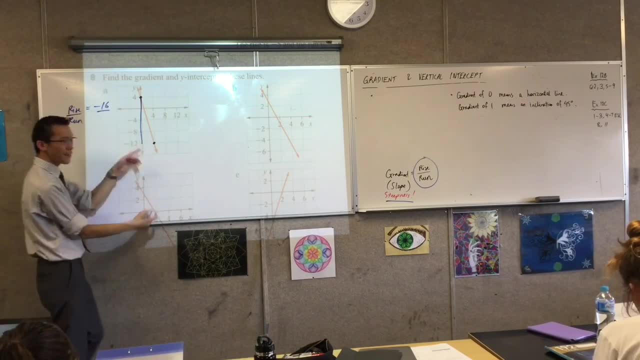 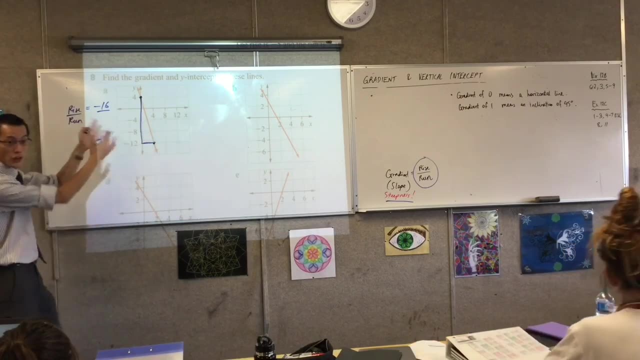 Okay, now I want to run. How far am I going here? Now? it's one square, but it's not one unit, It's actually four units. Watch out for that. You've got to read carefully. So that is the rise over run. 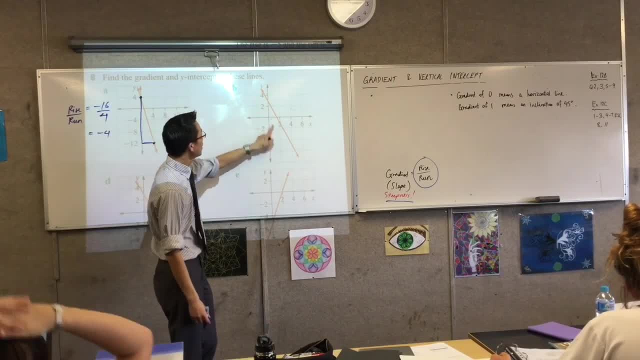 Now, that was an easy example. Other ones are not so simple. right, Look at this: The numbers. nothing's nice on the grid line, okay, But you still have to pick a point. I can still do it. Have a look at that. 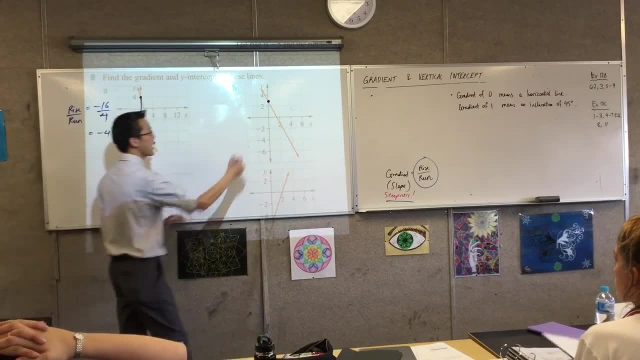 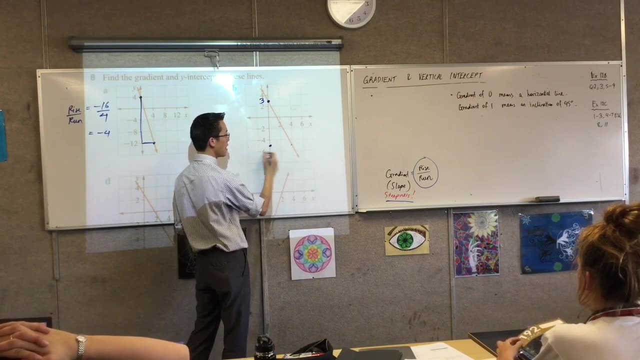 Halfway between 2 and 4?? That's 3, right. And in the same way, if I went to say New York, That's going to be halfway between negative 4 and negative 6.. So negative 5.. 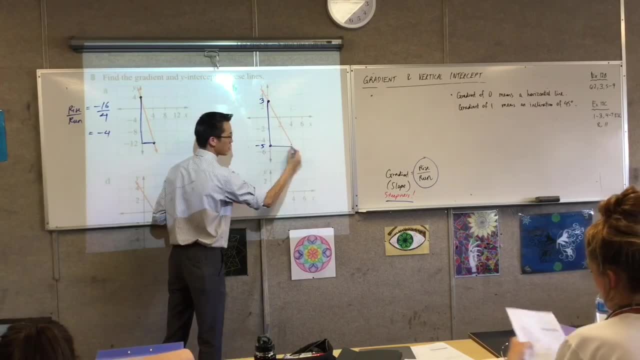 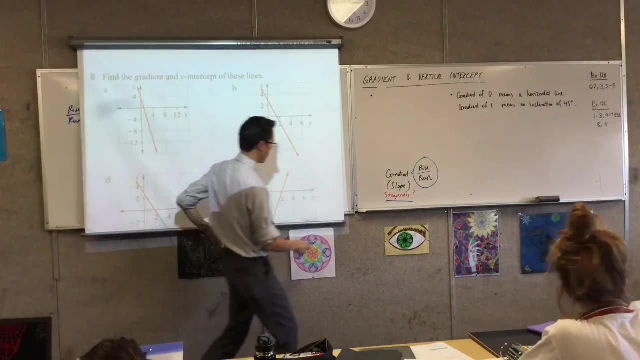 So I can still calculate the rise and I can still calculate the run. It'll all come down. Now one more thing I wanted to show you, And I want you to turn back to where you wrote this: The gradient of 0 and the gradient of 1.. 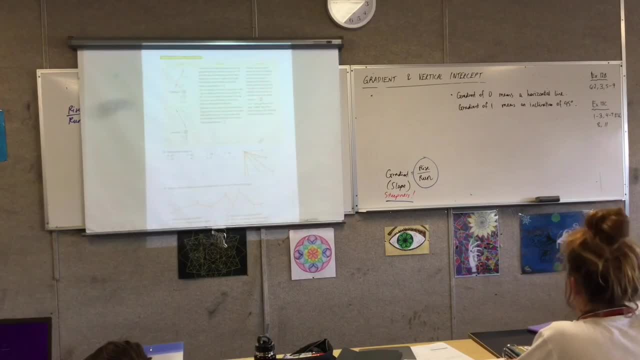 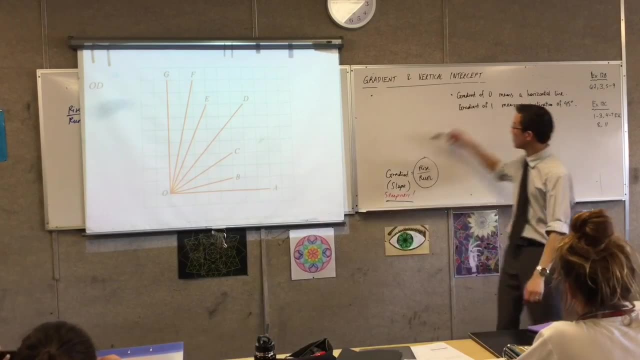 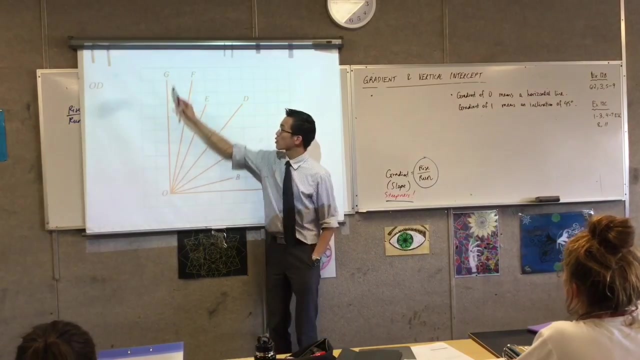 Okay, Now I just want to add one more thing onto this set of important results that you need to know. I hope you've done this question already. In particular, what I want to focus on is this: OG, bone, Now OG. 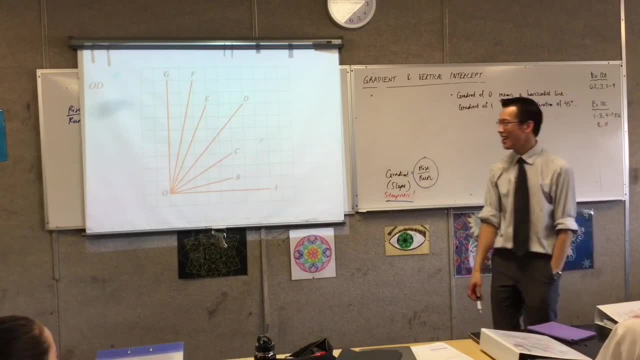 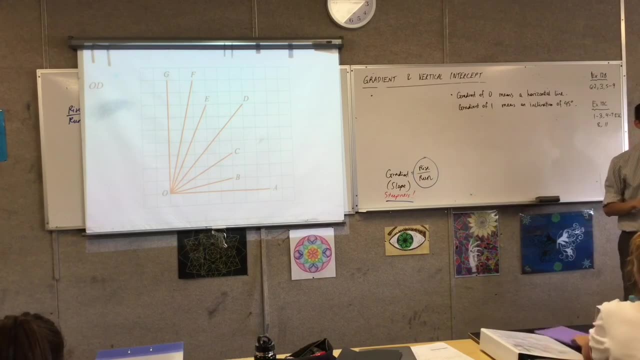 Sorry, say that again. Okay, now this is exactly the question I want to stress. Okay, And I have just the right amount of time to do it. So stay with OG. I'm sorry, what did I say? Stay with OG. 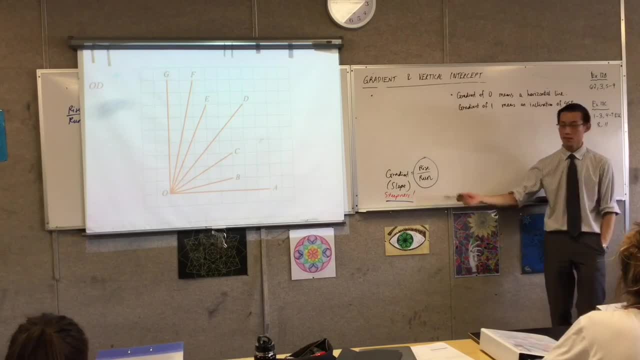 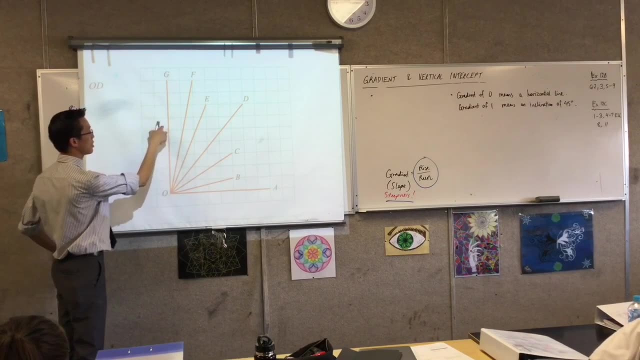 OG is a bit of a pickle, right, Because when you try and do this, rise is no problem. Rise is no problem. What is the rise? How many does it go through? 12?, 12?, 2,, 4,, 6,, 8.. 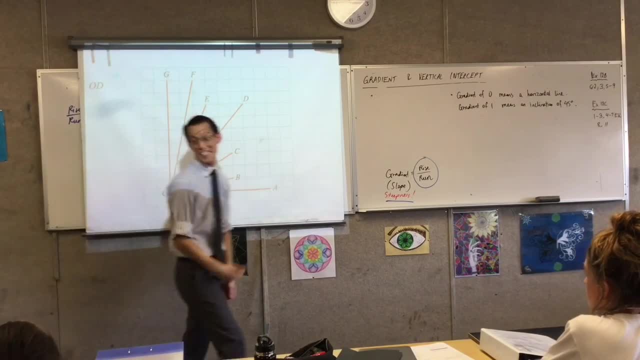 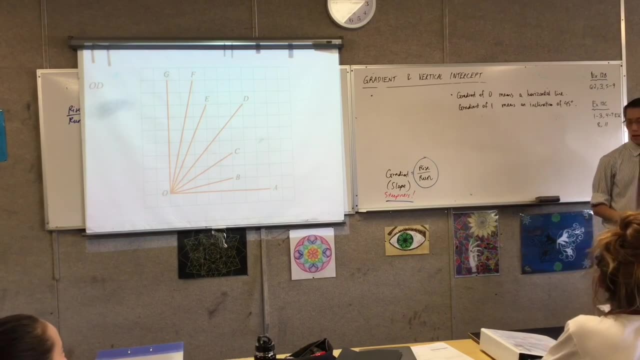 Wait, I just made it 9.. 9? Just a made-up number. Thanks a lot, Akio. Sorry, If rise is 9,, how far does it run? Zero? Zero, It runs zero. Okay, now this is a problem, because if I say 9 over 0, what is that? 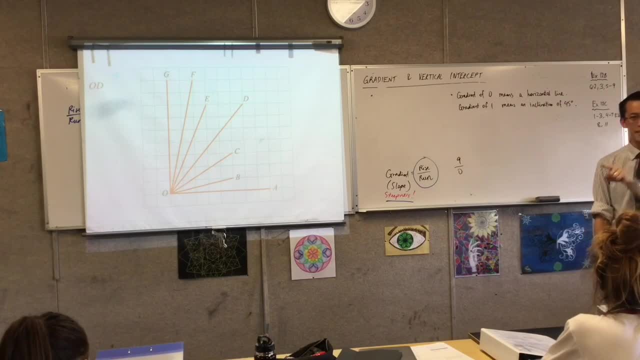 Zero. Now let me make a case for what it isn't Okay. I don't think we can say it's zero. The reason why is because I know what a gradient zero is supposed to be. It's supposed to be no rise. 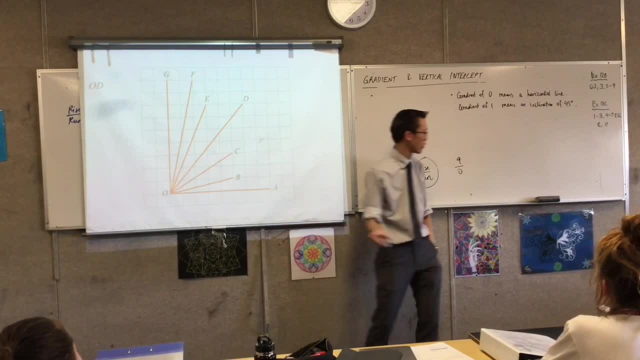 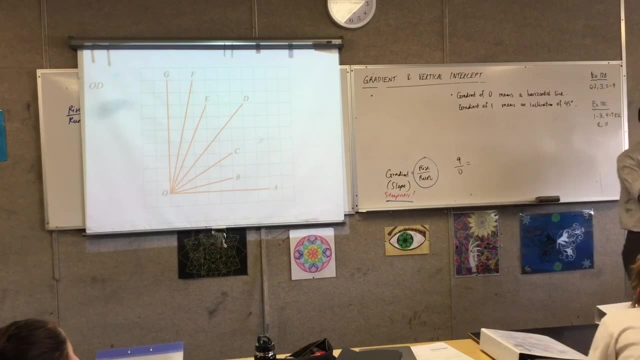 It's this guy down here, right? Do you agree with that? That's gradient zero. So, whatever this is, it's non-zero. So let's just play around. So let's just play a bit of an experiment. This is the whole point of algebra, right? 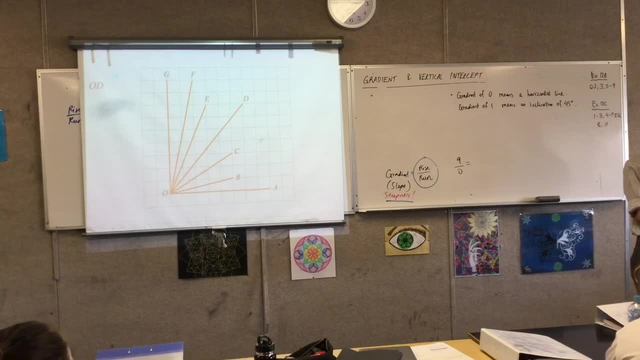 When you don't know what something is, you just give it a name and then you see what happens. Let's call it x. Now. a division statement like this is similar to a division statement like this: What's 6 divided by 3?? 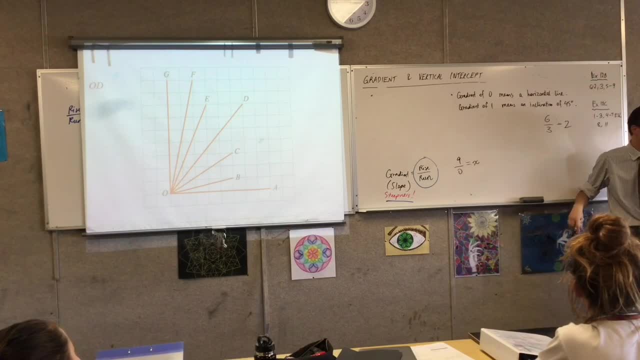 It was a long day, but your brain is still working. That's good. Now, the reason why we can say this is because I can multiply both sides by 3, and it's still true. Do you agree with that? So x equals 2 times 3.. 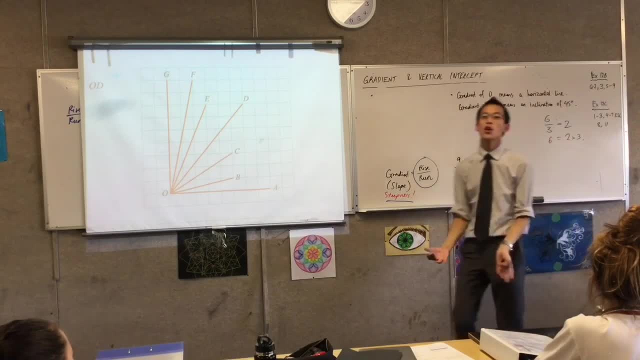 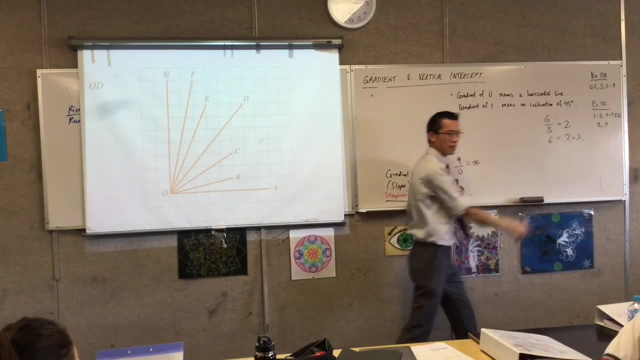 Does that make sense? Now look down here, Remember. I don't know what 9 over 0 is. I'm trying to work out what it's supposed to be. I've just called it x. If I can do this over here, I should be able to do the same thing here, right? 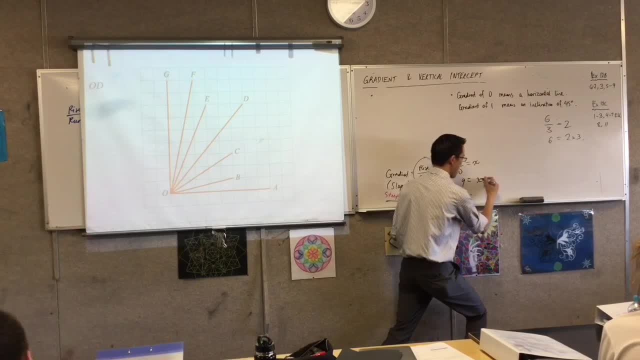 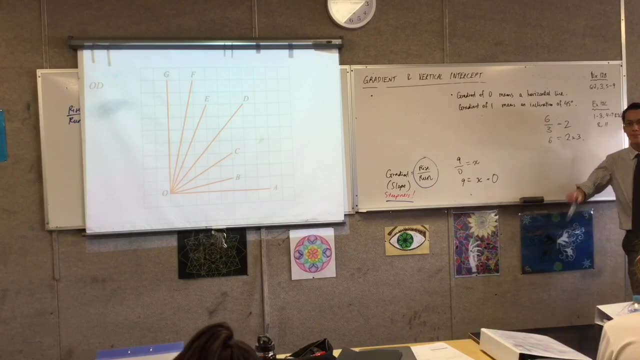 So 9 should be x times 0.. Hold on, I'm in trouble. Why am I in trouble? Because anything multiplied by 0 is 0.. The one thing we know about 0 is you multiply anything by 0.. 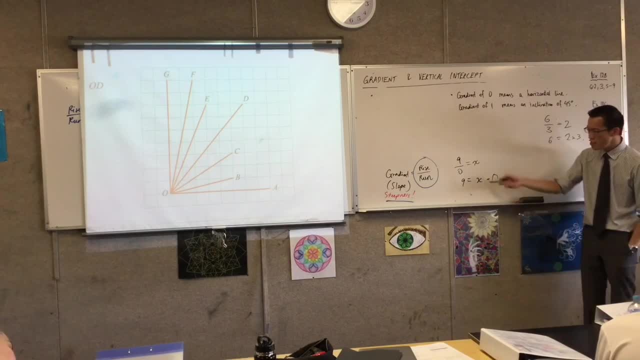 The one thing we know about 0 is you multiply anything by 0. You get 0. There is no number in the world. you can stick into x so that you get 9 at the other end, And that is why we say that this is undefined. 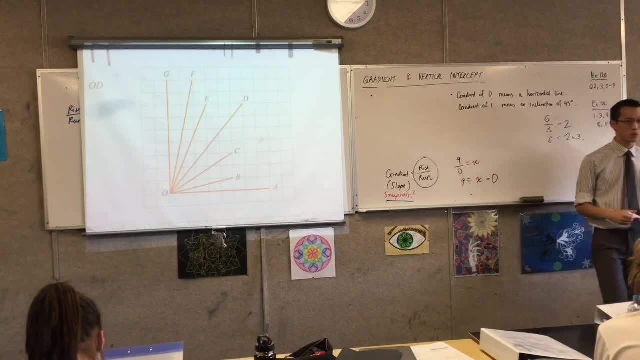 Your calculator will sort of spit the dummy out of you. Therefore, this is what I want you to add: right underneath here You've got a horizontal line right. Og is a vertical line, The gradient of 0 means a horizontal line. 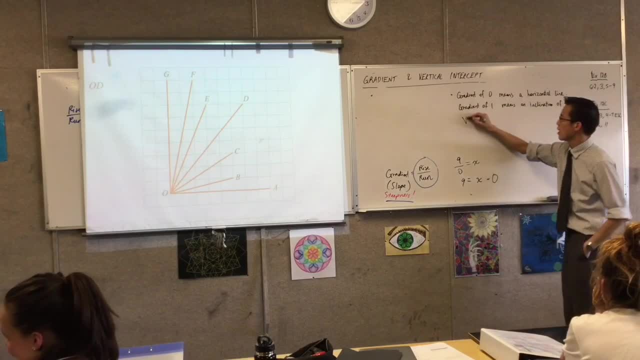 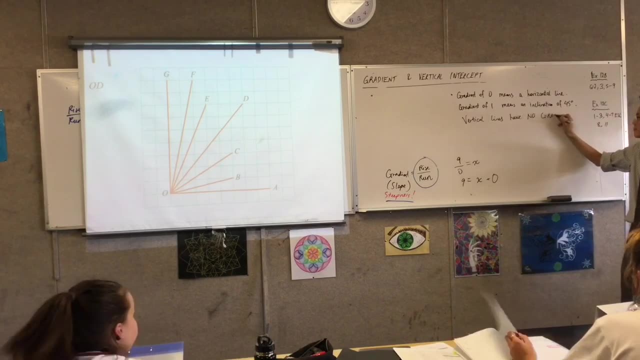 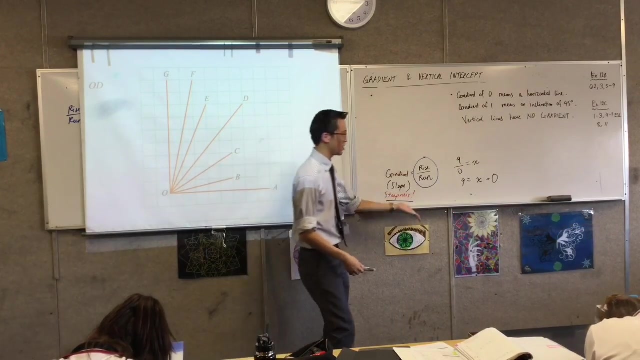 The gradient of 1 means the inclination of 45 degrees vertical lines. they have no gradient. they can't have a gradient because there's no run. you can't divide by zero, not because, like some math, god decided. we just wrote this down. 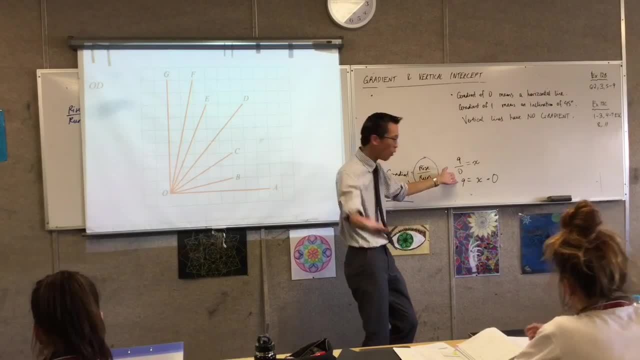 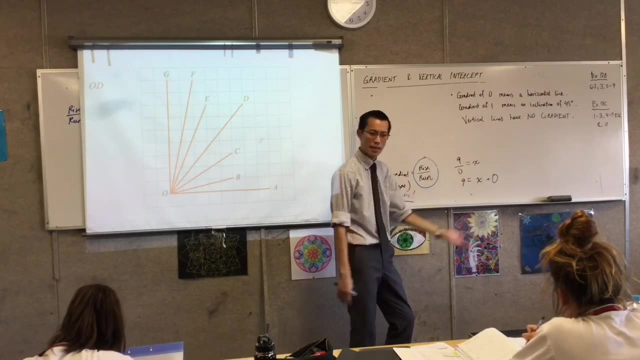 and everyone has to do that from now on. it's because the logic tells you. you all said to me that this should be zero. it can't be nine. nothing you can put there makes it nine. so x can't be anything. that's why we call it undefined and it doesn't have a gradient.